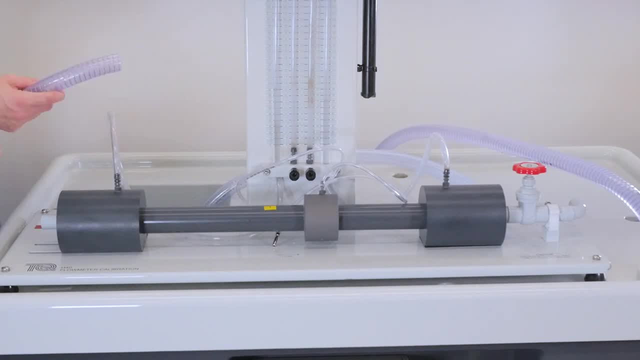 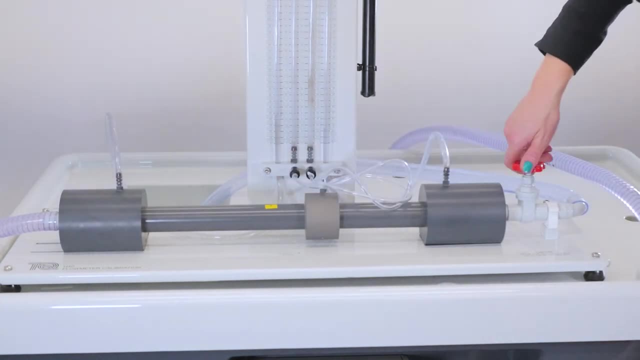 application, Whether it's a civil engineer working on rivers and canals, a mechanical engineer working with flow pipes and conduits, or marine and aerospace engineers. And as with many things, there are trade-offs. Some devices are cheaper, others easier to fit, and there are 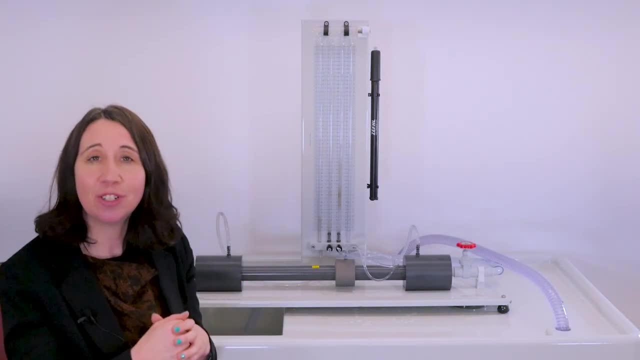 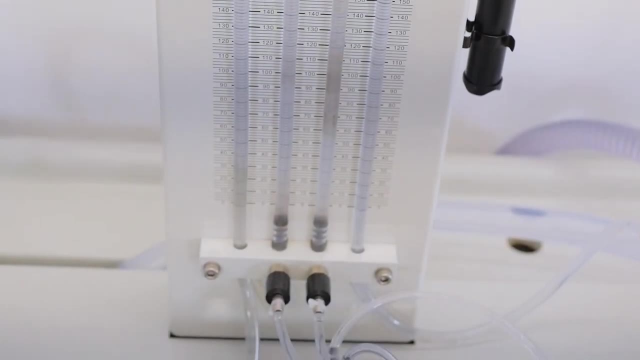 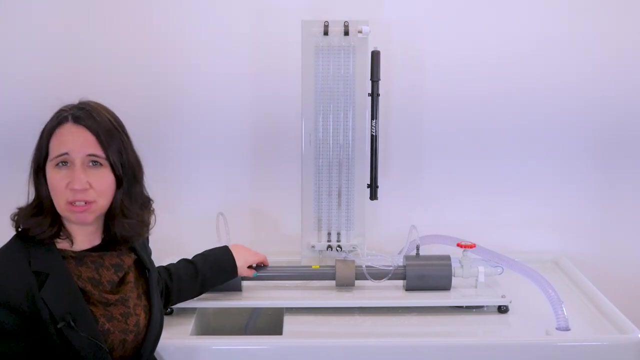 varying levels of accuracy, ranges and losses. Let's take a closer look around the apparatus. We have a back plate and stand and on the back plate there is a set of four water-filled manometers That show the pressure differences of the flow meter and across the overall flow meter section. 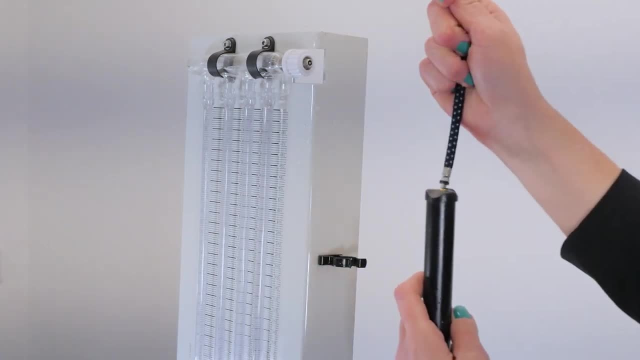 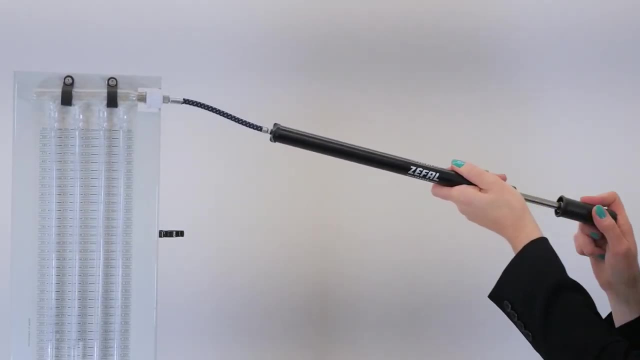 At the very top, here is an air valve. The air pump on the side is easily removed and connects to the air valve in the manifold. The pump can increase the pressure in the manifold to allow the level of the water to be adjusted, enabling the pressures to be read effectively. 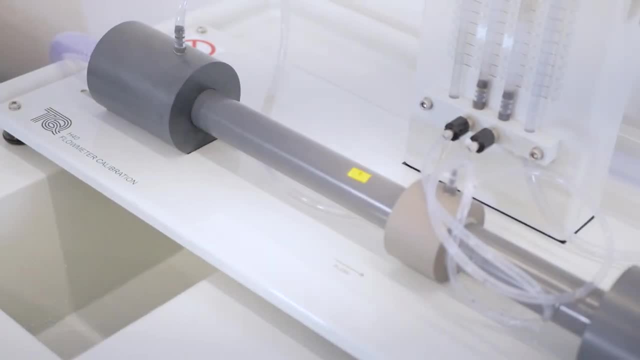 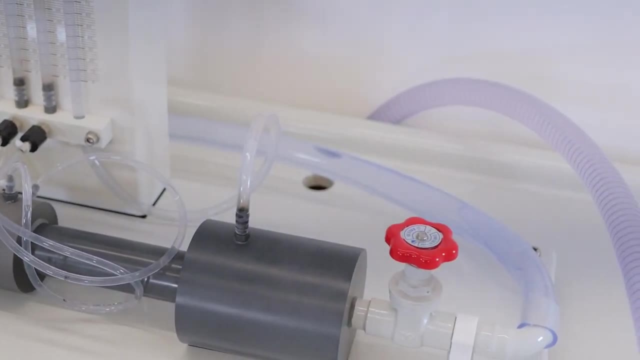 Down to the stand there is a water inlet and outlet connection. We're using this with Tech Equipment's hydraulic bench so we can connect up the pipes like this, allowing you to measure the flow rate. It also provides a mobile water source and drain that can be positioned anywhere in the 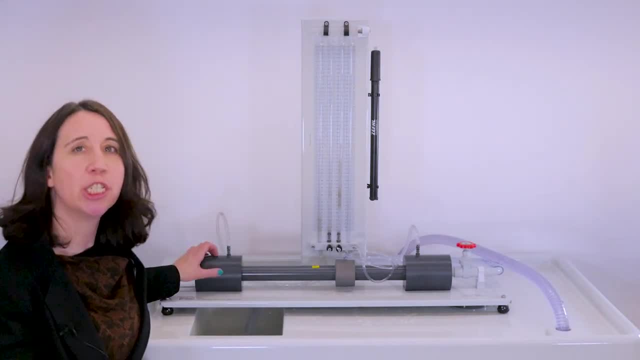 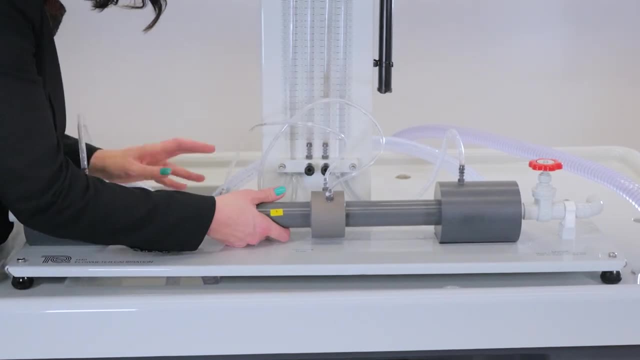 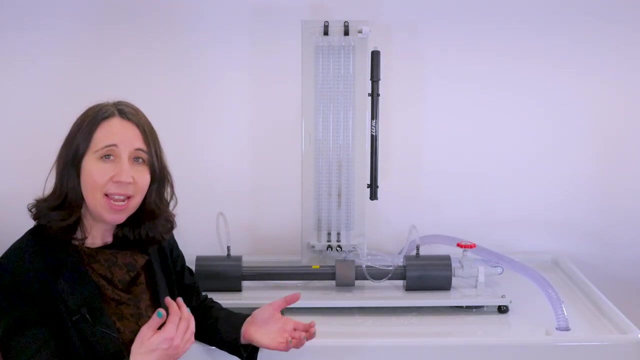 lab. These chunky sections on either side of the connector blocks allow you to easily switch over different types of flow meter by sliding them into place. As you can see, it's simple, and the sockets and seals ensure there is a tight fit for no leakages Inside. these are two water-filled pipes. 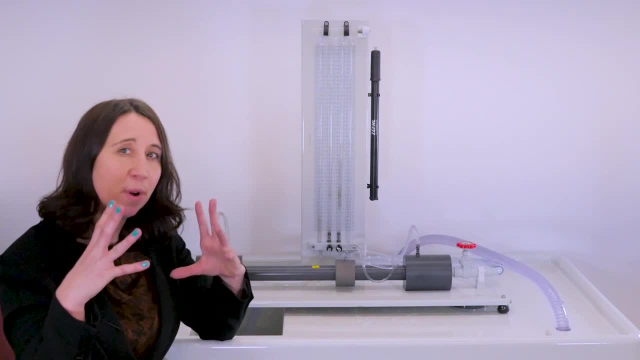 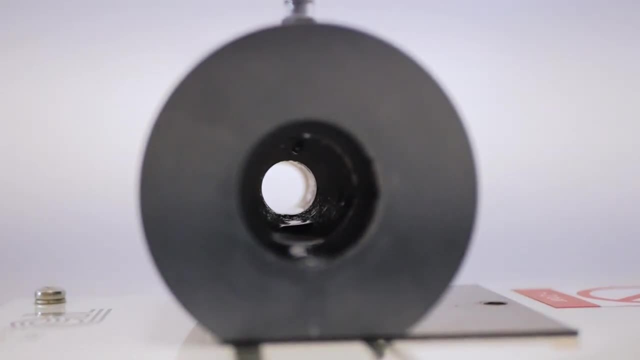 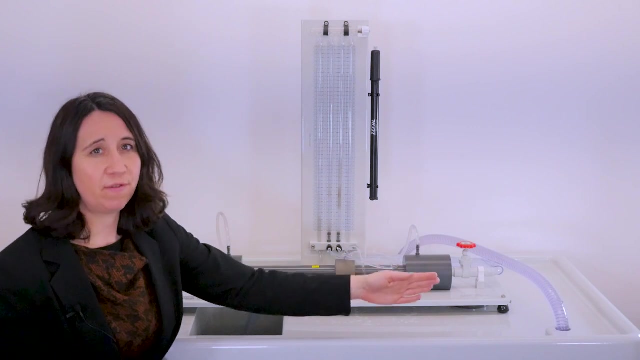 Inside these there is a gradual expansion of the internal bore on the inlet and gradual contraction of the internal bore on the outlet to reduce unwanted flow disturbances. Now to look at the outlet, which has a gate flow control valve that controls the downstream of the water flow. The pressure measurement connections have self-sealing push fit connectors. 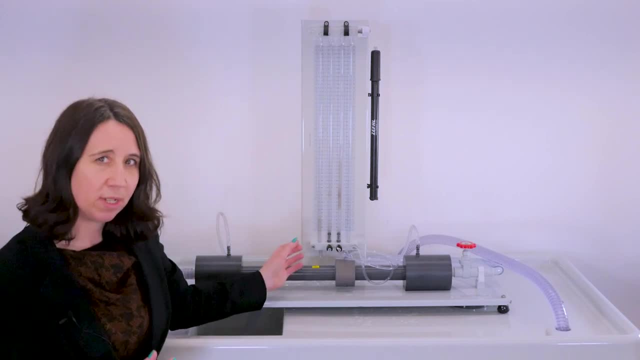 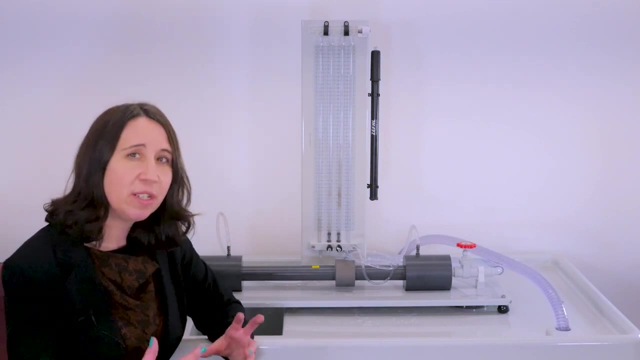 Let's take a closer look now at how this works. Cold water passes through the flow meter. The second and third manometers show the pressure drop at the flow meter. The other two manometers show the total pressure drop across the inlet and outlet, measured at the adapters.